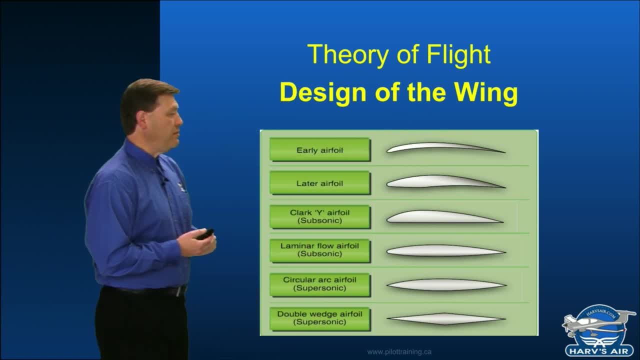 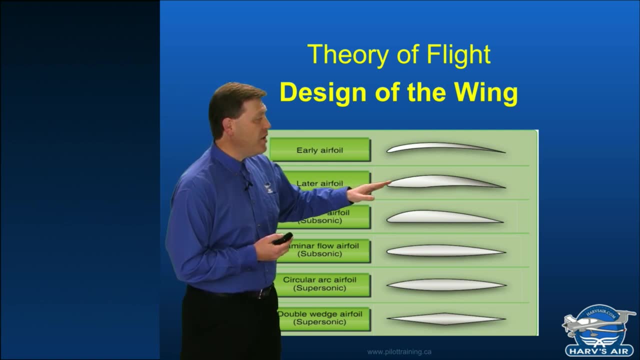 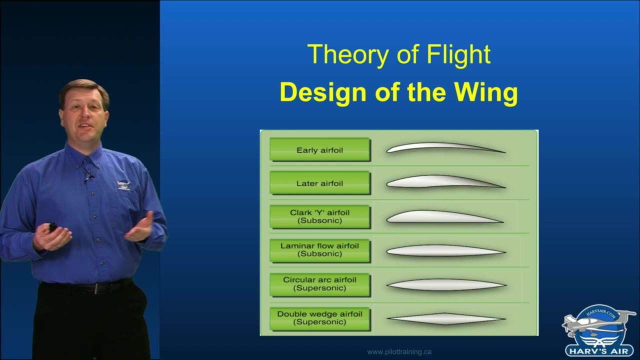 That's going to generate lift upwards. Later on, we see that we actually ended up with an airfoil that became a little more straight along the bottom And slightly more curved on the top, And then, as we started to design faster and faster airplanes, we discovered that these had certain deficiencies. 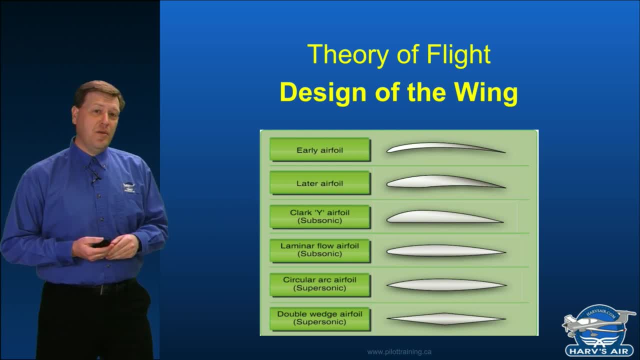 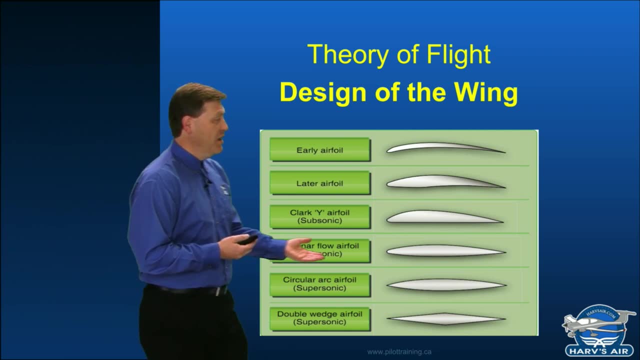 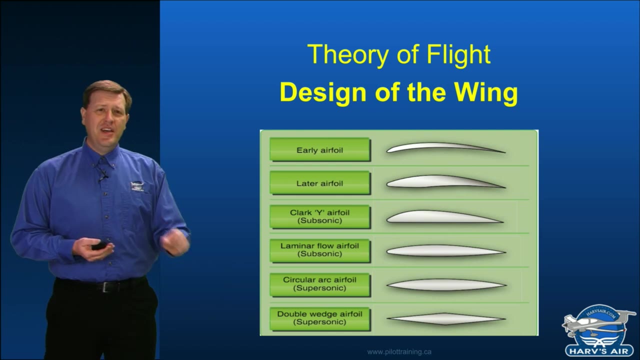 And we started to work more and more towards what are known as laminar airfoils, And those gave us laminar airfoils. So we'll start to take a look at some of these individually later on, But let's start out first with the overall wing plan form. 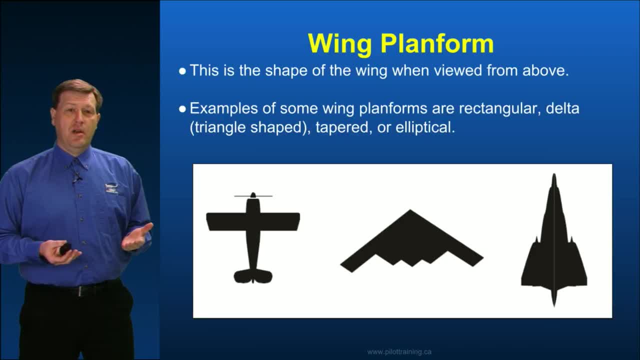 When we talk about wing plan form, we're asking ourselves: what does the wing look like from the top? So you can see over here to the left we've got a fairly rectangular looking wing, Almost like a chocolate bar. In fact, sometimes these types of wings here are referred to as the Hershey bar wing. 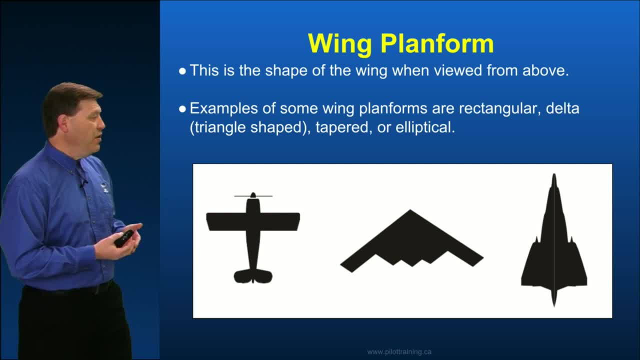 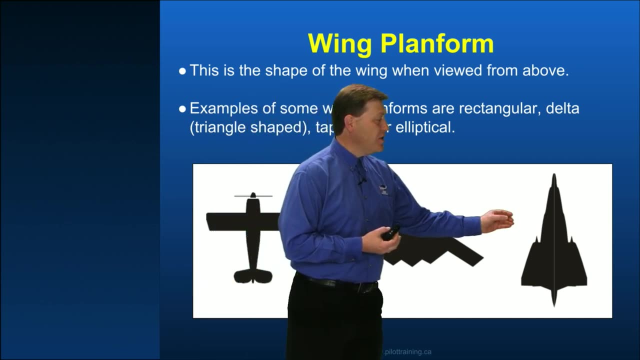 Because they look like a Hershey chocolate bar. Over here we've got more of a kind of combination of a tapered wing And as well, a triangle shaped wing, And then finally over on the far right when we start to look at some really, really fast aircraft. 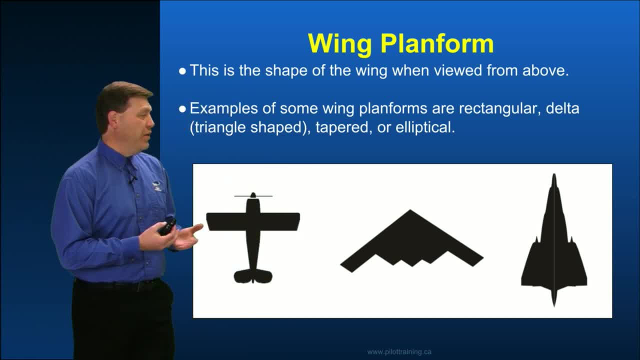 we've now got the delta wing. Now, as we move on, we're going to start to see that there's benefits to a wing like this. But then there are certain situations where a rectangular wing isn't going to work very well, So we're going to want to move more over towards the delta wing. 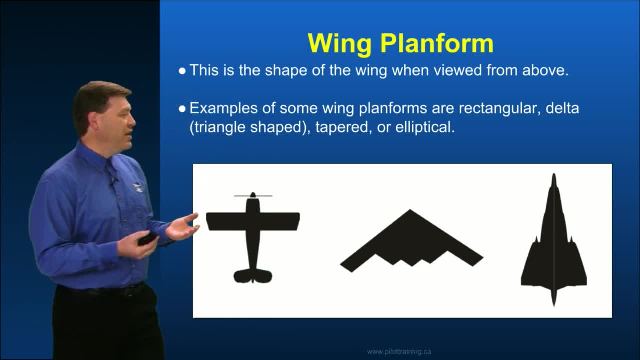 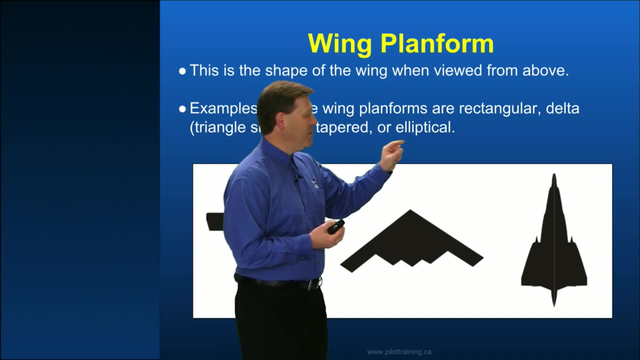 But you know what? Perhaps actually I'll start out with the white board And start to show you some of the various plan forms and how they affect our airplane. Oh, shouldn't, don't forget the tapered elliptical. I almost forgot to mention that one. 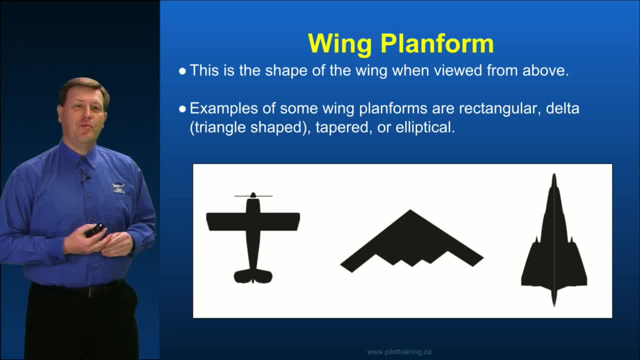 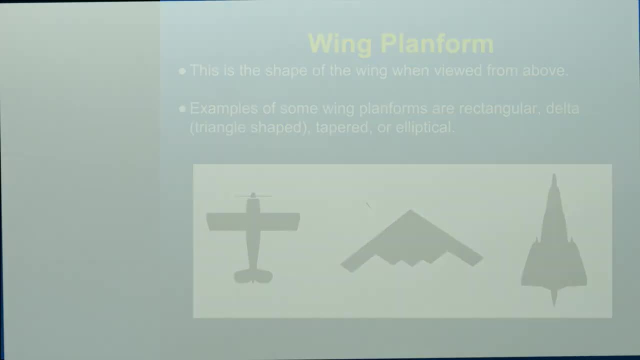 That's actually sometimes referred to as probably one of the most perfect wing designs in existence. You know, the Spitfire from World War II, an elliptical wing. It has some very good qualities, But let's go over to the white board and start to draw out some of this. 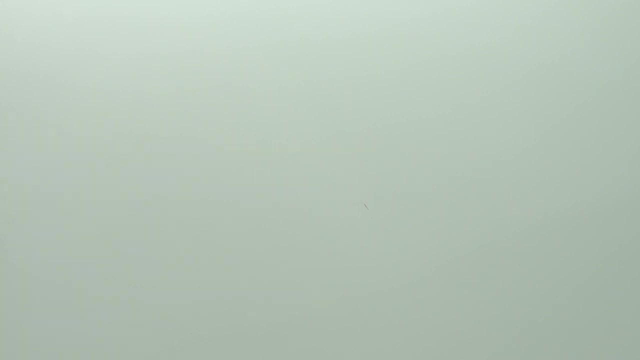 When it comes to the wing plan form- particularly so when we think of GA airplanes, the trainers that you're going to fly- we could start out with, say, a rectangular plan form. So that would be like the chocolate Hershey bar wing. 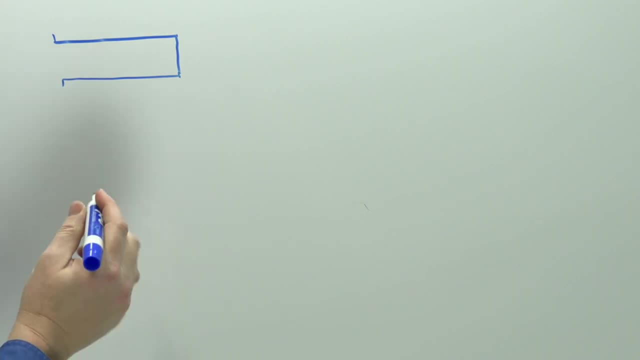 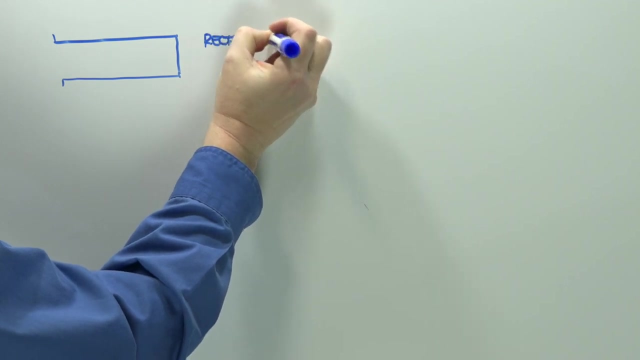 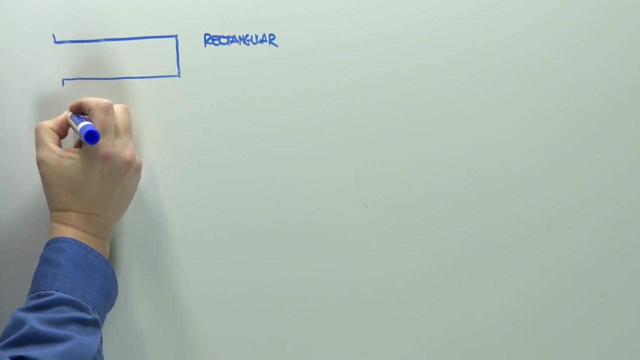 So, of course, over on this side we've got the fuselage. We could also end up- let's call this, of course, you know the rectangular. But then we've also got what are known as tapered wings. Now, that would be a wing, perhaps where from the fuselage. 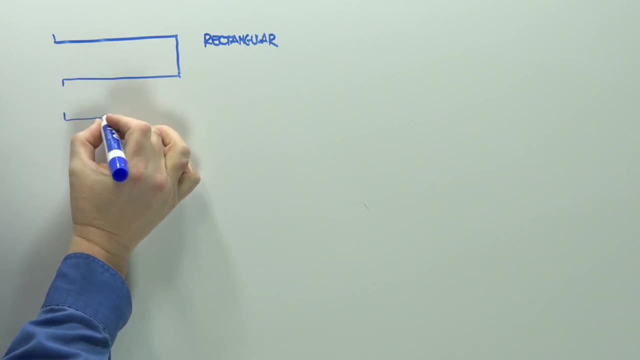 it might end up, you know, starting out fairly straight, But then it will have at some point maybe a taper to it. This is, say, a later version of that Of a warrior wing. So just draw that fuselage here. 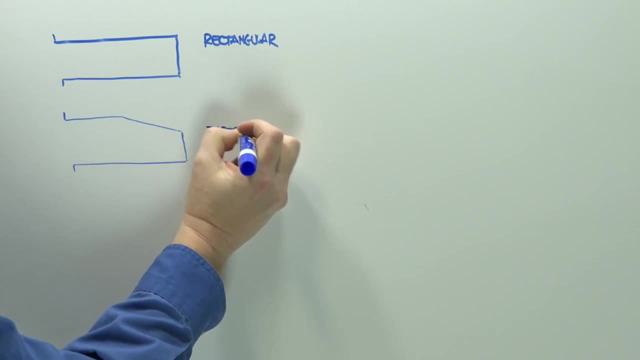 So this is tapered, And then we've also got- perhaps we could call it the elliptical, which isn't used very often anymore. So this would be as I mentioned on the Spitfire wing. I'm just going to draw in a set of ailerons here for each wing. 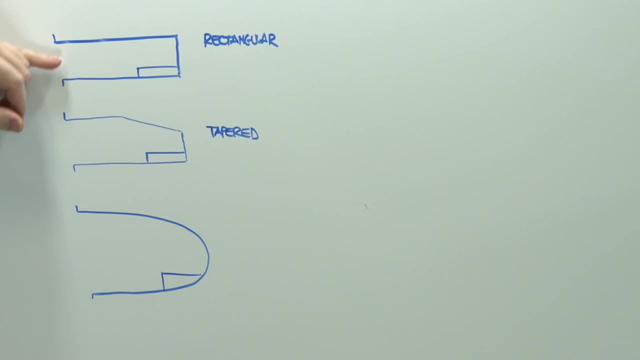 And then let's talk about how and why engineers will choose each one of these types of wings. What they found is that each of these types of wings actually has different stall characteristics. The rectangular wing: what it will tend to do is it will tend to start to stall in here, near the fuselage. 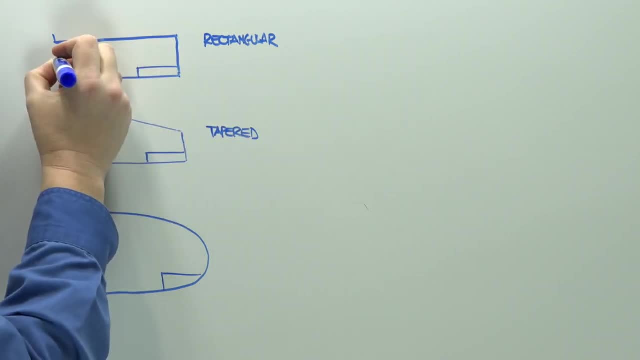 And as we get slower and slower and slower, what will happen is that region of stall will slowly spread outwards from the initial stall near the root, So it will head out there and then it will continue out here as you get slower and slower. 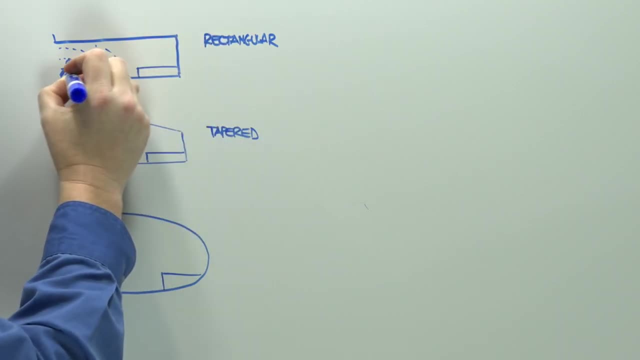 So it will stall from the root outwards With a tapered wing. the stall characteristics change A tapered wing. what it will tend to do is it will start to stall in this region here Then, as we continue to slow the airplane down. 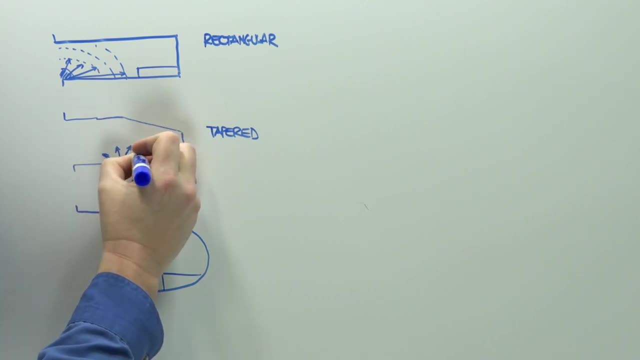 that region of stalling will spread outwards like that, So you'll end up with this being the stall area and then this being the stall area. over time. Now, an elliptical wing stalls very differently. What it actually does is it stalls at the very, very trailing edge, initially. 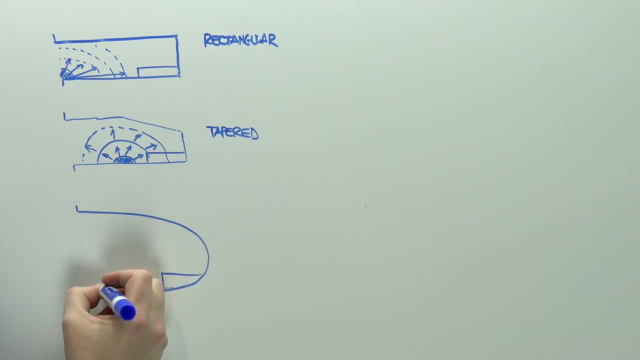 So in that zone, And then, as this airplane gets slower, it will continue to stall, moving from the trailing edge forward. So it will look like that and eventually like this and eventually like that. So that's how we end up with the typical stall pattern. 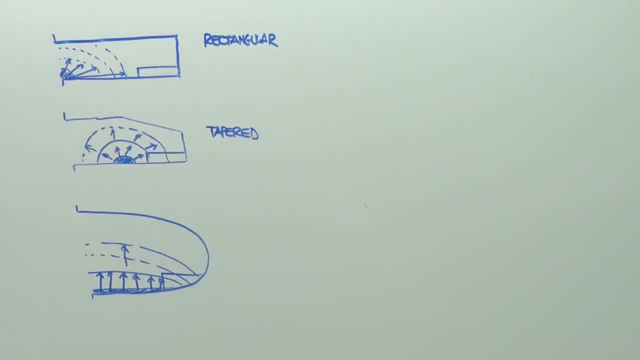 of each of those plan forms. Now, as we look at each of these plan forms, imagine you're flying a training airplane. Well, the tapered airfoil isn't quite as nice, because what will happen is eventually the ailerons become inside of that stalled zone. 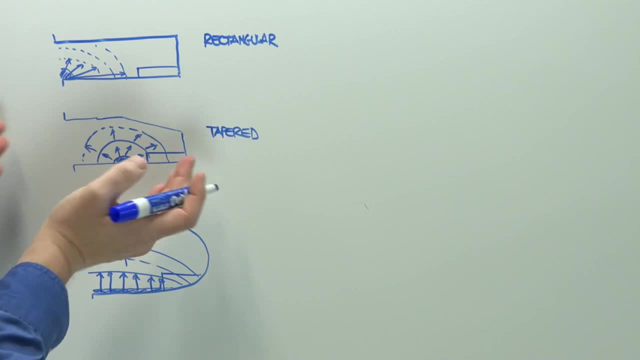 So what's that going to do for our control As we approach the stall? we're not going to be able to control our aircraft. The elliptical has sort of the same problem as well, But take a look at the rectangular wing, Because it stalls near the root. 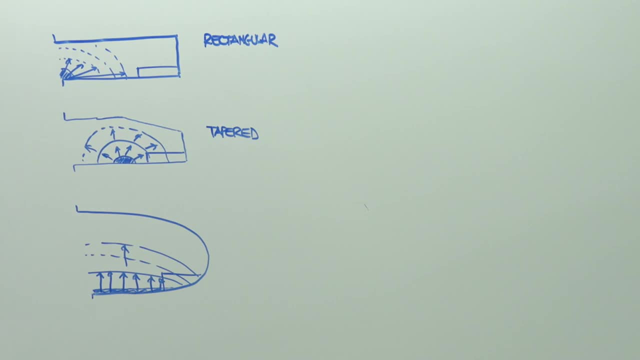 one of the last things to stall happens to be the ailerons, So we're going to have good control all the way up to the stall. Now, you'll see later on in the presentation that there's some tricks that we can use to actually cause the tapered wing. 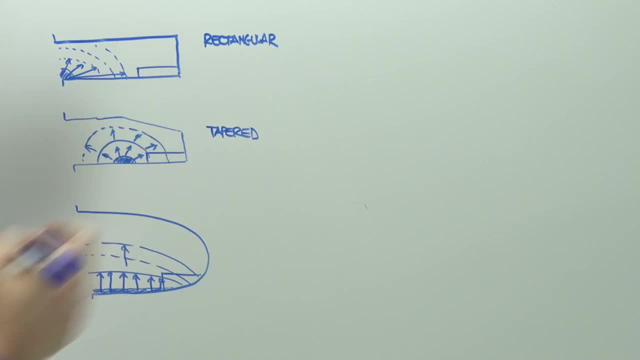 to not stall at the ailerons so early. It's known as washout. Now this isn't immediately obvious, but let's start to now think about, say, some of the drag characteristics of these air or plan forms. As I look at the rectangular airfoil, 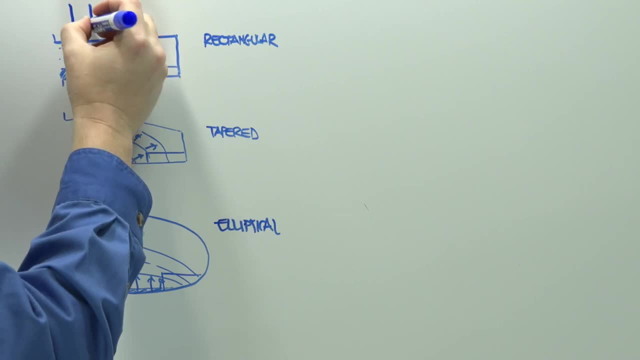 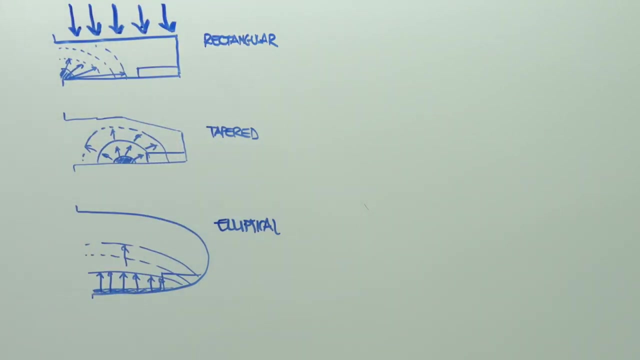 well, imagine the air flowing towards the rectangular airflow or the rectangular airfoil, the leading edge of this particular wing. I can see that, you know, at every point the airflow is directly perpendicular to the leading edge. So these are going to generate